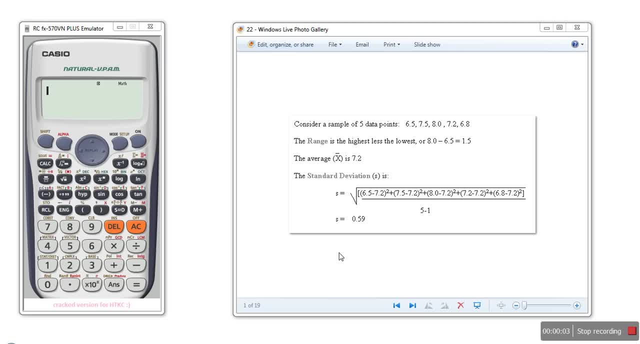 Hello everyone, In this video I will show you how to calculate average standard deviation and variance. For this exercise I have taken this example. We are having sample of 5 data points and this is a solved one. We also solve it in our calculator. So first of all we need to set the mode. 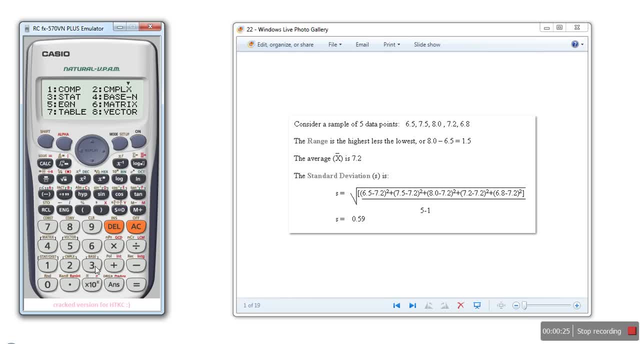 Press MODE key and select STAT MODE And in this value select variance by pressing 1.. So here enter your data. So we are having this data. So we will enter 6.5 equal 7.5 cosine, then 8, then 7.2.. 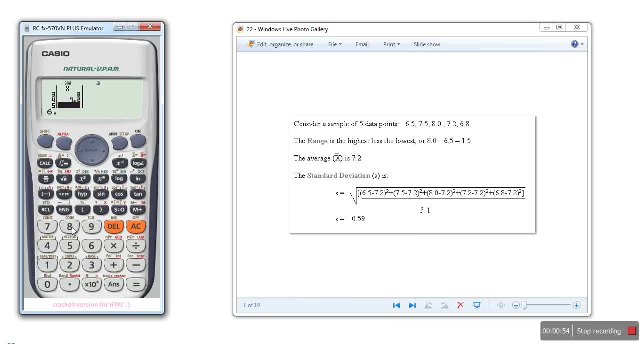 And finally 6.8.. So once data part is done, enter AC key So it will save your data in memory. Next thing, what we want to calculate. So we will press SHIFT key and then we will go in STAT MENU. 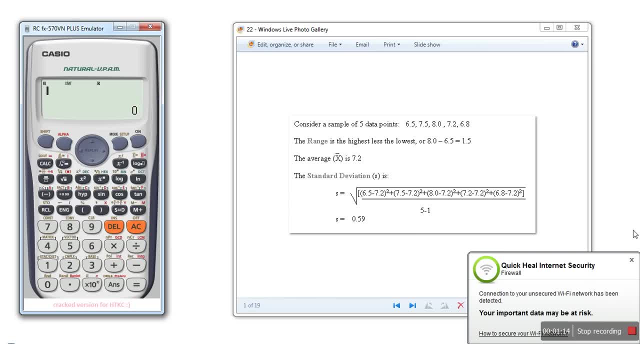 If you can see, here STAT is written on the key 1.. So we will press 1.. So it is asking what we want. So it is asking what we want. So it is asking what we want, So we are going for variance 4.. Press 4 key. 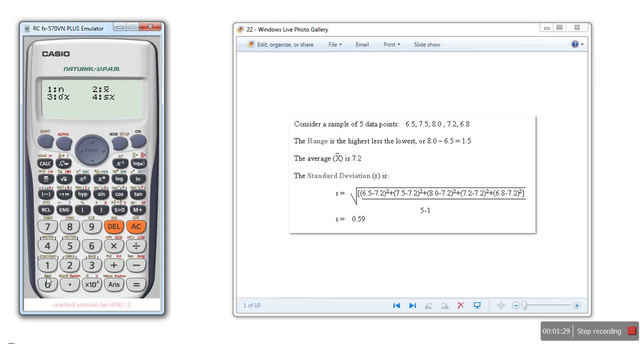 So here, M, if you press 1, this will give you the total number of data points. X bar, this will give you the average Rho, X it will give you variance, and SX it will give you standard deviation. So first we will calculate X bar, So we will select 2 and we press equal key. 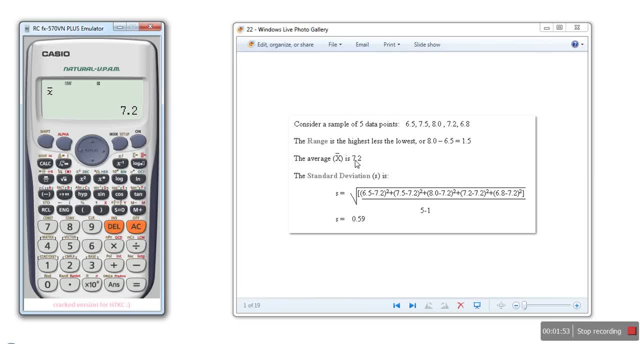 So 7.2, this is the average And if you can see, 7.2, this is the average of this data given in this example. Now we will go for standard deviation. Again, we will go in MENU VARIANCE. 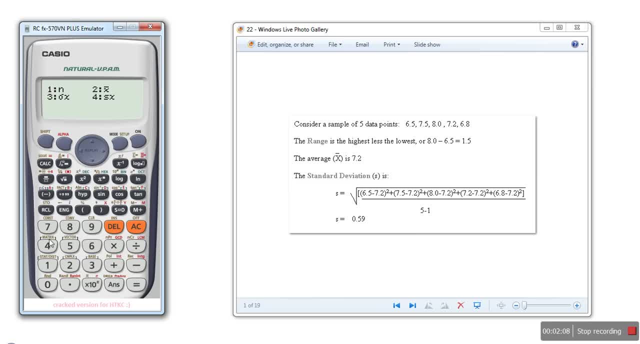 So for standard deviation, SX 4, equal sign. So standard deviation is 0.58736.. So in this example they actually truncated the output to only 2 digits. So in this example they actually truncated the output to only 2 digits.